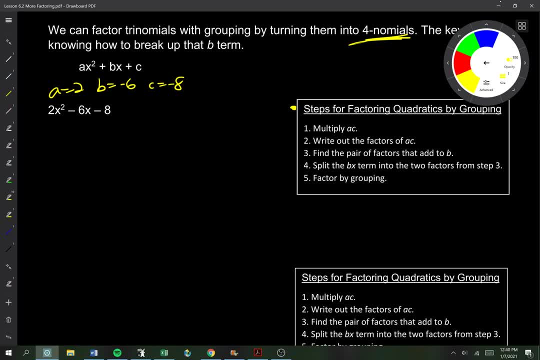 steps for factoring by grouping. I'm going to follow these steps. It's fairly straightforward. actually It's a lot of steps, kind of, but they don't take long to do. The first step is: multiply a times c. a times c is 2 times negative 8, which is negative 16.. I'm going to 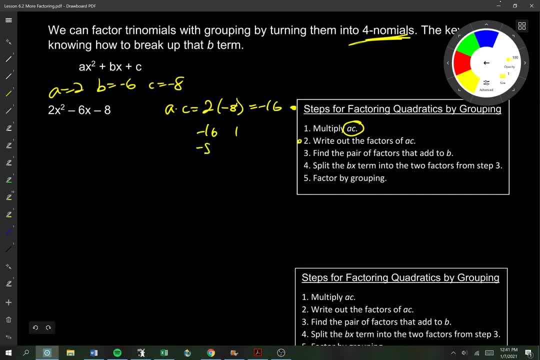 next, write out the factors of negative 16.. I recommend you do this in a really organized fashion, like 16 divided by 1,, 16 divided by 2, 16 divided by 4, and then don't forget that if you 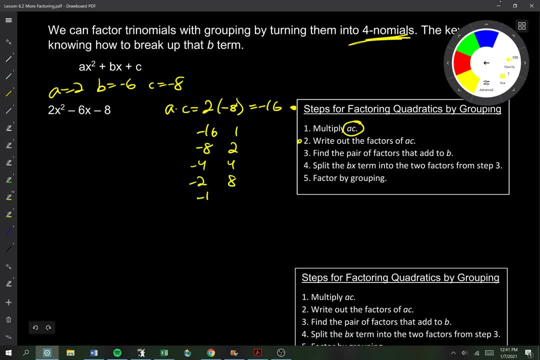 have negative 8 and 2,, you also have negative 2 and 8.. If you have negative 16 and 1,, you also have negative 1 and 16.. Okay, that was step two. Write out the factors. Step three is to find the. 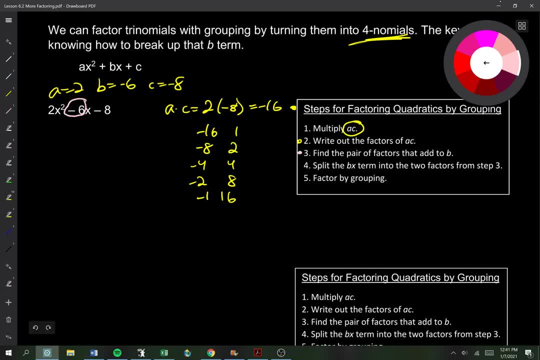 factors that add to b. I want to find something that adds up to negative 6.. Negative 8 and 2 add up to negative 6.. So negative 8 and 2 are the two values I'm going to get that I split this b term, So bx is going to split into the two factors that I just got. What 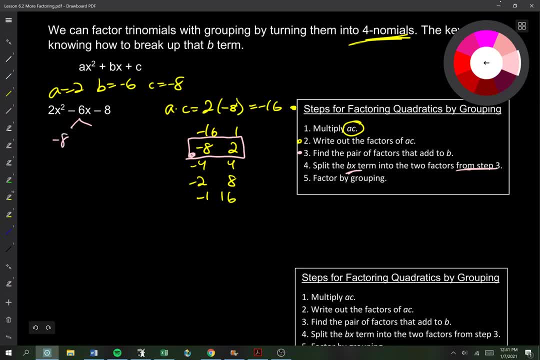 that means, is this negative 6x is going to become negative 8x plus 2x. The minus 8 and the 2x squared are still there And I have now made a four-term equation. I'm going to get a four-term expression out of this three-term expression And it's a very special four-term. 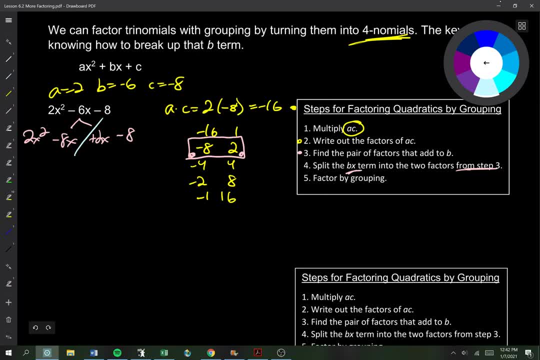 expression because it can factor Out of the left half. here I can pull out a 2x, leaving me with x minus 4.. Out of the right half, I can just pull out a 2,, leaving me with x minus 4.. These two things will combine into one bubble, one factor, And these two combine. 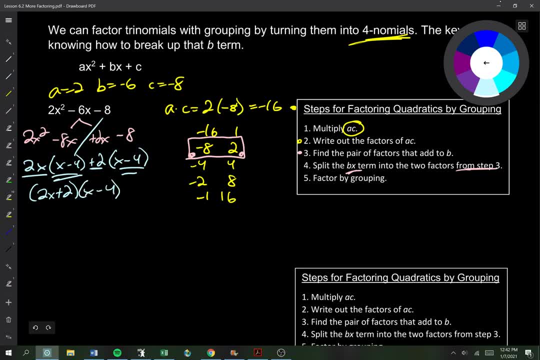 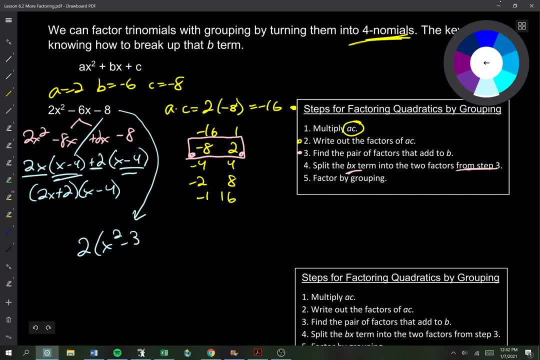 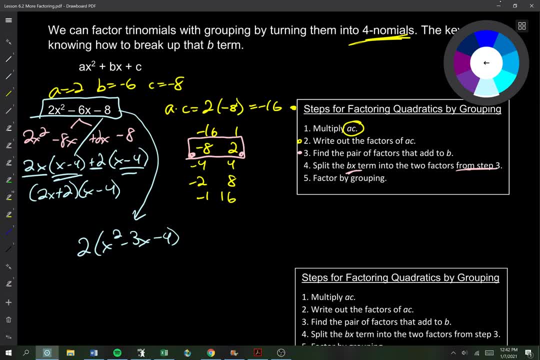 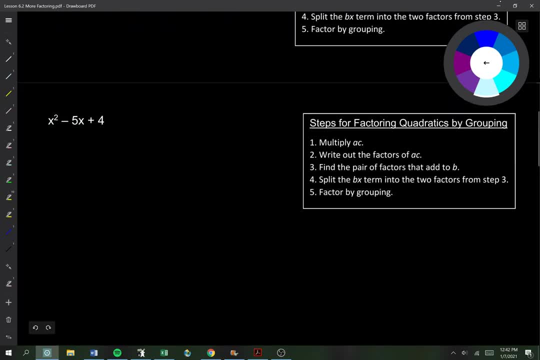 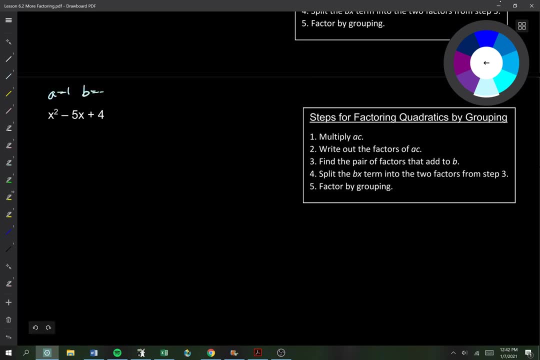 that out. We'll talk about that more in a future video. So this is factoring by grouping. You follow these steps, You factor by grouping. It's fairly straightforward. Let's do another example. I have x squared minus 5x plus 4.. Well, my a term is 1. My b term is negative. 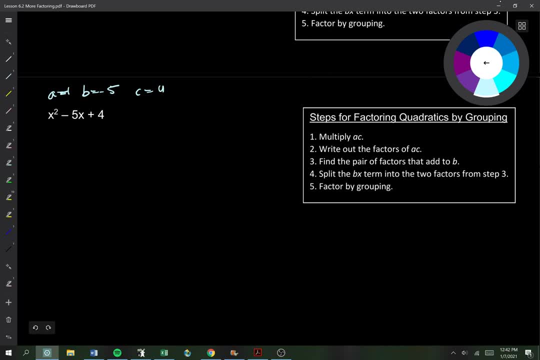 5.. My c term is 4.. I multiply a and c 1 times 4 is 4.. And I write out the factors of 4. and there aren't that many. Don't forget negatives. Negatives count as factors here. I want to find the. 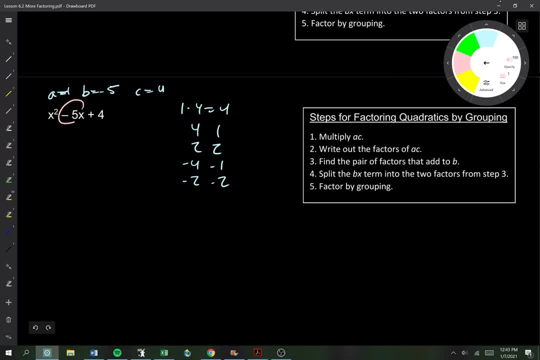 pair of factors that adds up to negative 5, because negative 5 is my b term And that's these two right here. So I'm going to split this up into x squared minus 4x, minus 1x plus 4.. You can flip the order of these. It doesn't matter which order these two terms come in. 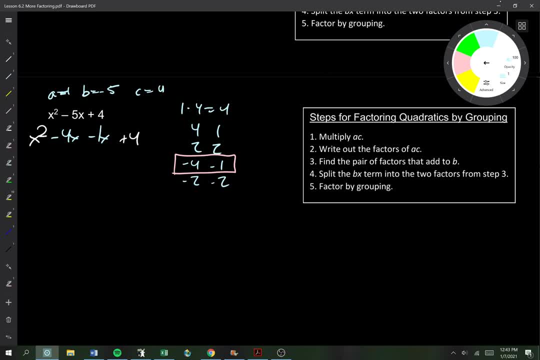 It'll still factor just fine. So either way you set this up is going to be okay. Now, on the left side of this, I can factor out an x And I'm left with x minus 4.. On the right side, all I can pull out is a negative 1.. But I do pull out the negative 1.. That again. 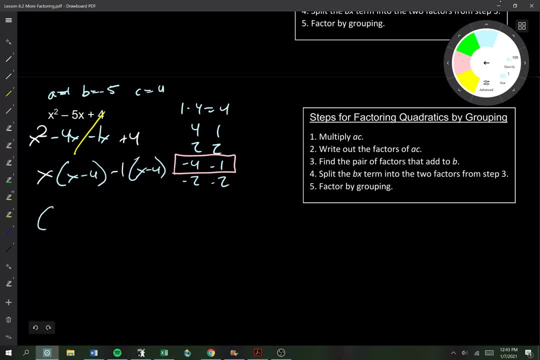 leaves me with x minus 4.. So I combine the x minus 1 and the x minus 4.. And boom, We factored. Remember the way you check factoring is: you go back and you do the redistribution again. x times x is x squared, x times negative. 4 is negative, 4x Negative. 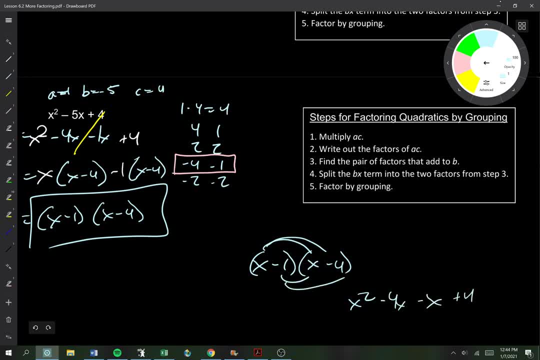 1 times x is negative, x Negative. 1 times negative 4 is positive 4.. This becomes x squared minus 5x plus 4, which is what we started with. So the check is solid. Okay, that's factoring by grouping. It will work every time If a problem cannot be factored. 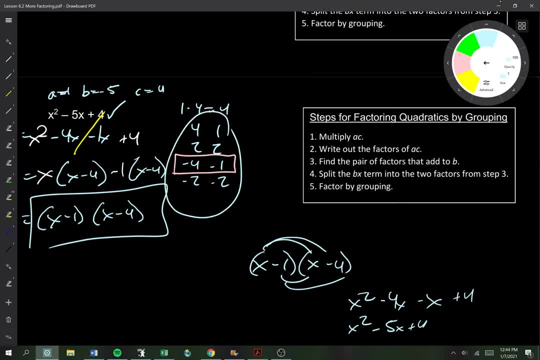 you wouldn't be able to find a pair of factors that add up to the b term. So you're going term like you need. So it'll tell you pretty early right here at step three. If step three is impossible, then you'll know the problem can't be factored like x squared plus x plus. 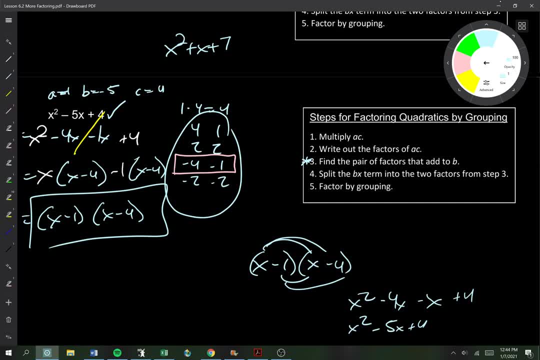 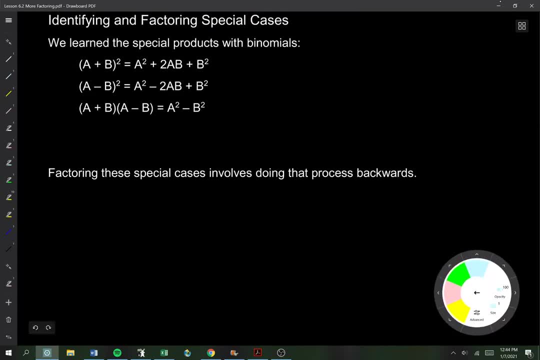 seven. That's a problem that can't be factored, and the grouping process will break down at step three. There's some faster ways to factor, though. Those are called special cases. Special cases we talked about with multiplying earlier in the year. You know, we know that a plus 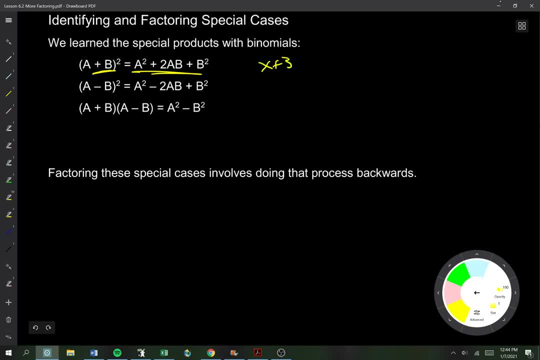 b squared equals a squared plus 2ab plus b squared, Like if I have x plus 3 squared, that is not x squared plus 9. It's x squared plus 6x plus 9, because you have to do x plus. 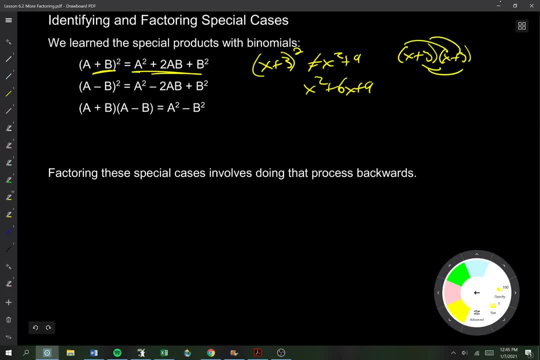 3 times x plus 3, and you have to do your foiling. So these are the three special products that we worked on last chapter: A plus b squared, a minus b squared. and then the difference of squares: a plus b times a minus b is a squared minus b squared, For example, like: 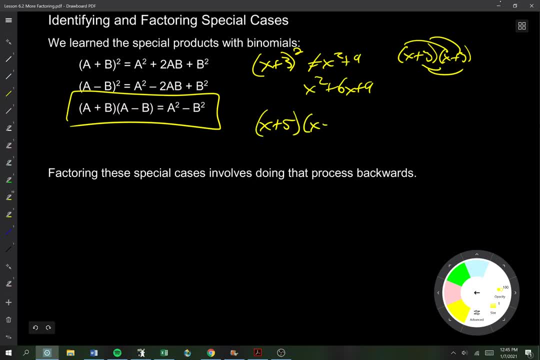 um x plus 5 times x minus 5 is x squared minus 25.. That's an example of a difference of squares. That's an example of a difference of squares. That's an example of a difference of squares. Well, factoring is just doing that process backwards If I have a perfect. 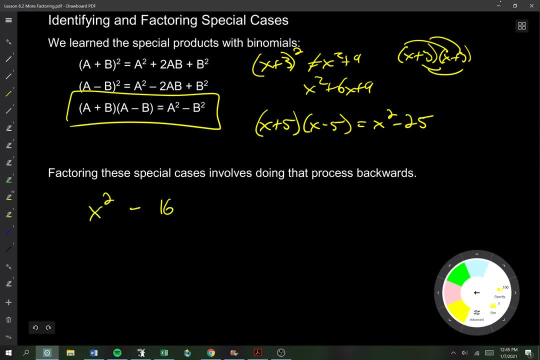 square and another perfect square and they're being subtracted. this is called a difference of squares and I know that can factor into the square roots, right? The square root of 16 is 4, so x plus 4 and x minus 4.. If you have two perfect squares that are subtracting. 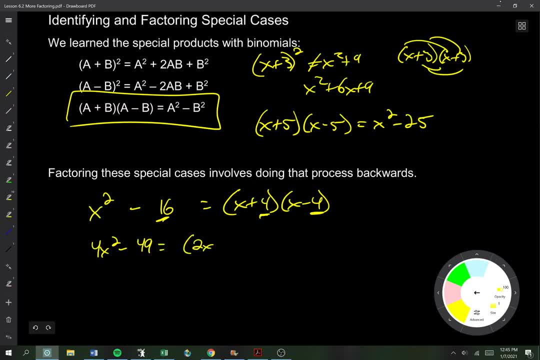 each other square, root them and put a minus in between them, And there you have your difference of squares. Okay, that's a special case that you can factor very, very quickly, and it's fairly common to have a difference of squares. It's something that pops up pretty frequently. 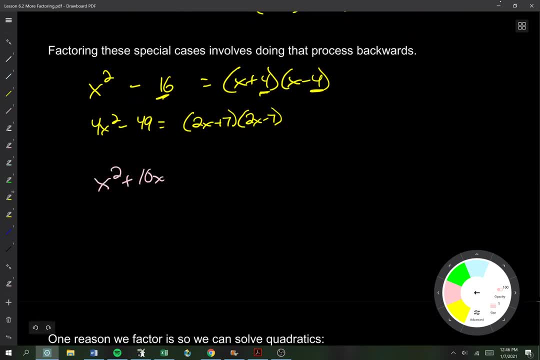 So another example is if I have something like x squared plus 10x plus 25.. Well, here's what I'm looking for: If my c term is a perfect square and my a term is a perfect square and my b term is even 2,, 4,, 6,, 8,, 10,, 12, something. 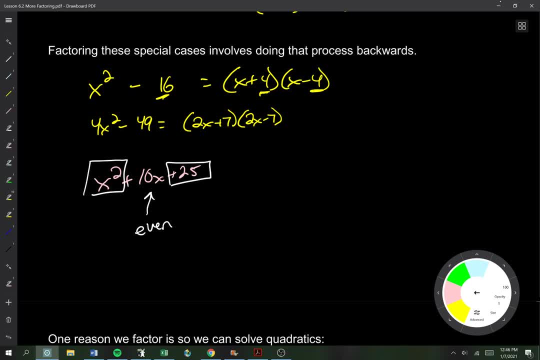 like that. If these three things happen, my a term and my c term are perfect squares. my b term is: even. then I think it's fairly likely that this factors into x plus 5 times x plus 5.. So I do it and I check it. You have to check it because that won't always. 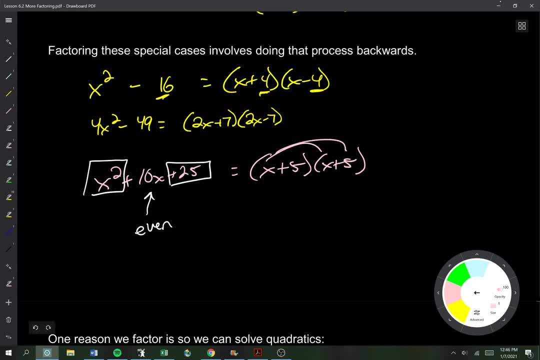 be the case, okay, But I get x squared plus 5x plus 5x plus 25.. So I get x squared plus 25, which is x squared plus 10x plus 25.. So, yes, it checks. So if your a term is a perfect. 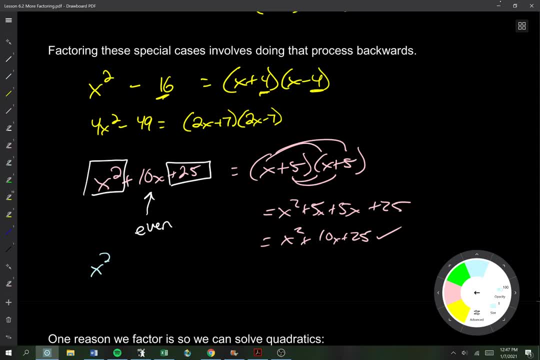 square and your c term is a perfect square and your b term is. even then, it's very likely- not guaranteed, but quite likely- that you have a special case. This would be x minus 10 times x minus 10, which we would just write as x minus 10 squared. 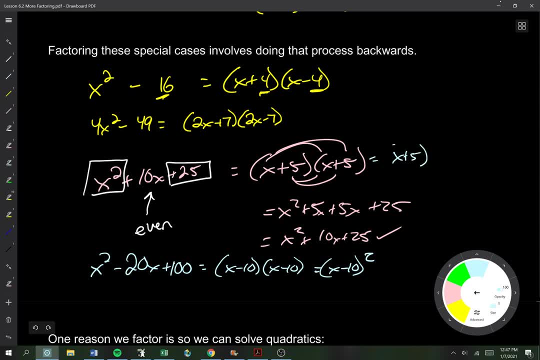 Like up here, we would actually write this as x plus 5 squared, because that's prettier And it's actually easier to work with If your a term and your c terms are squares and your b term is even positive or negative. but even it can probably factor by this special. 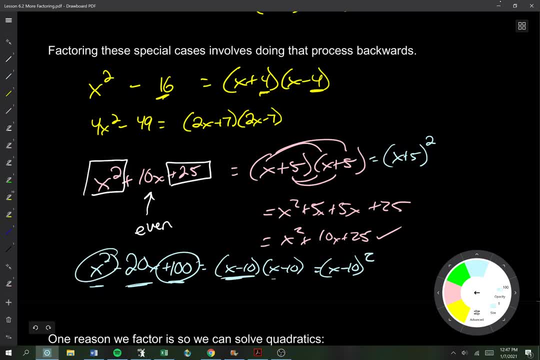 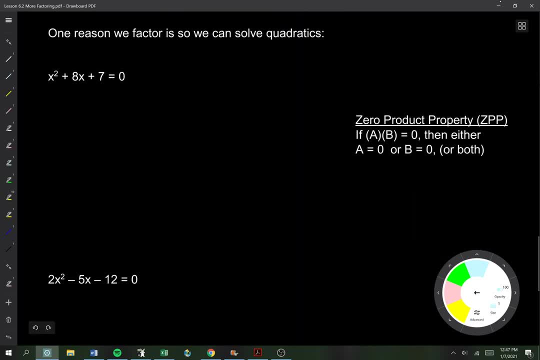 case where you square root this and square root this and make them both minus or plus, depending on if it's subtracting or adding the b term. Okay, finally, the main reason, not the main reason, one major reason that we solve or that we sorry. 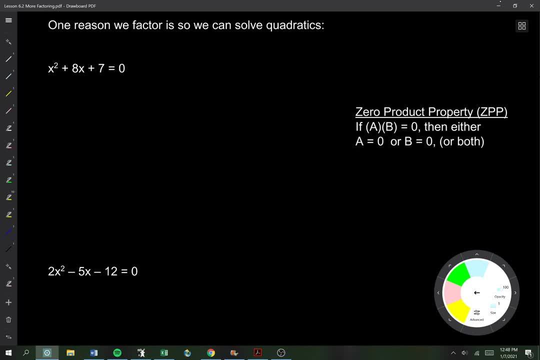 Okay, finally, usually I edit these videos, but I'm not going to because I'm tired and out of time, So you just have to live with me clearing my throat like that, I'm sorry. A major reason that we factor is so we can solve quadratics. It's not the only reason. 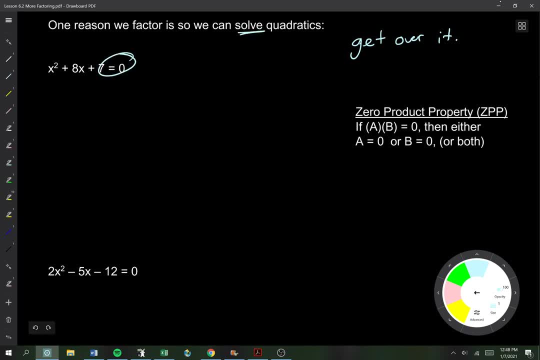 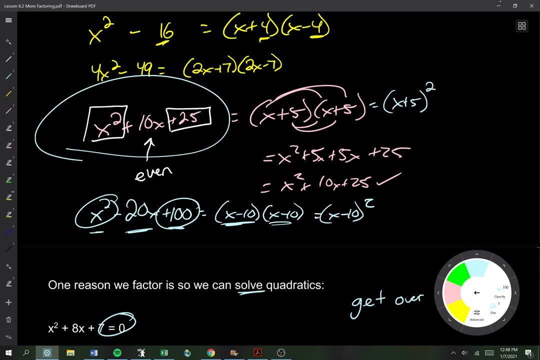 but it's a major reason Now. solve means you have an equation. So far we haven't had equations right, Like these weren't equations, These are just expressions. We were factoring, We were rewriting in different forms. This is an equation made of two expressions. 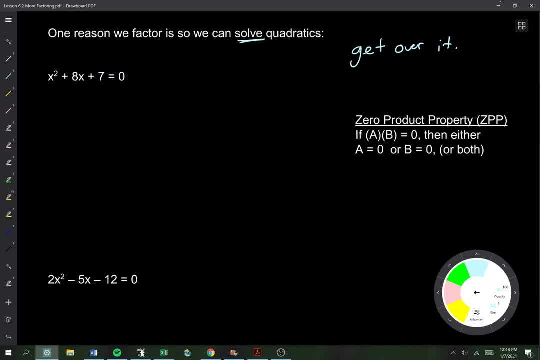 We're going to take the quadratic expression and factor it, and then we're going to use the factors to solve. See, we're trying to find the values of x that we could plug in. Like, what numbers could we plug in for x? so this comes out to zero. Well, if you try, 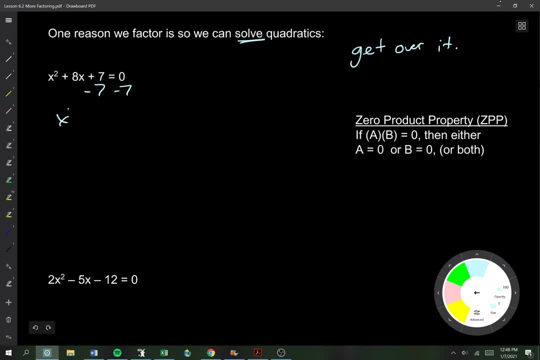 to solve this by regular algebra methods, where you like. just try to get the x by itself. it doesn't go very well because you have two x's, Like. if you divide everything by x, you get x plus 8.. 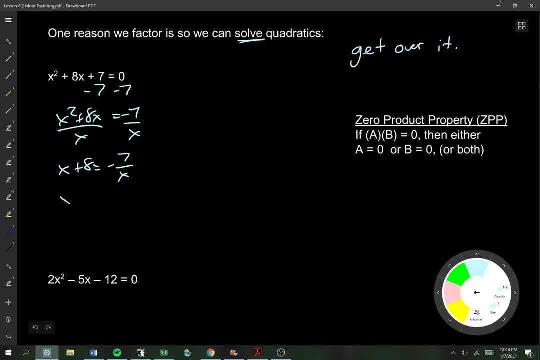 It equals negative 7 over x, and then maybe you subtract the 8 from both sides, but you have an x here and an x here and it's not going to go well because you have multiple x's. But one option is to factor. This can factor into x plus 7 times x plus 1.. Okay, 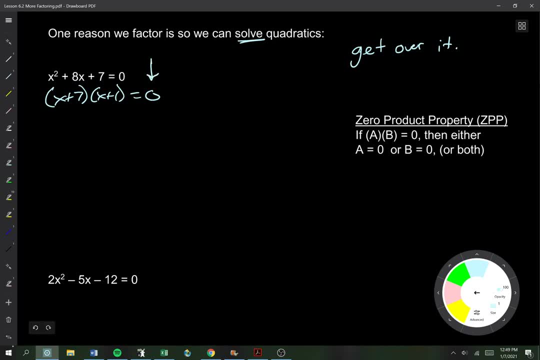 that's how that factors. The key is that it's equal to zero. If something is equal to zero, we can typically apply what's called the zero product property, which basically states: if two things are multiplying to zero, one of them must be zero, And possibly they both. 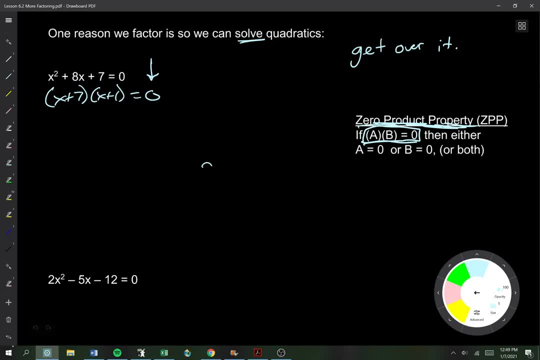 are, but at least one of them has to be zero. See, if we have 3 times something equals zero, we know that, that something is zero. And if we have something times something equals zero, we know that one of those something is zeros. But that's only true with zero. If we have 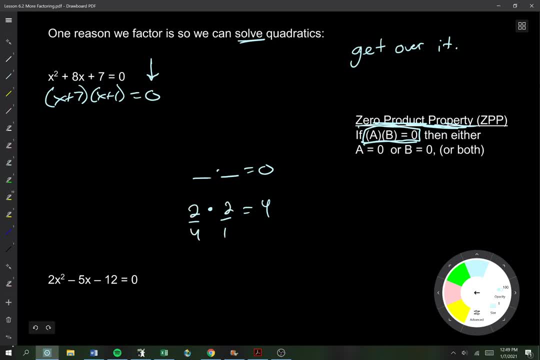 something times something equals 4, it could be 2 and 2, it could be 4 and 1,, it could be 8 and a half. There's an infinite number of things, an infinite number of pairs that can multiply to 4.. But if you're multiplying to zero, we know that one of them must be. 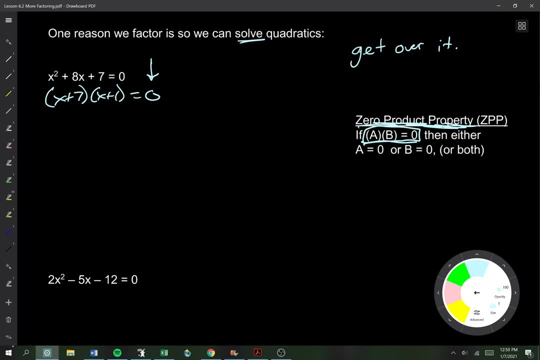 zero. That's called the zero product property. So basically, when I have this equation- x plus 7 times x plus 1 equals zero, I know that either x plus 7 equals zero or that x plus 1 equals zero. So I solve both. These are my solutions. 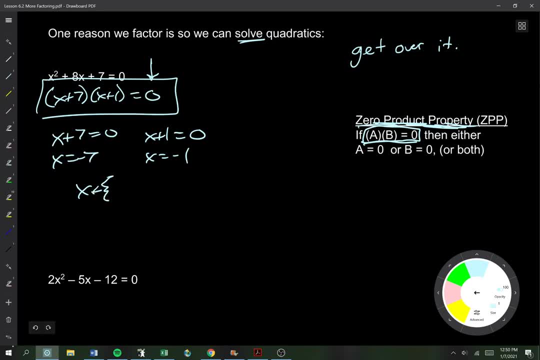 We could say: x is the set of negative 7, negative 1.. You factor and then, once you've factored, you solve your two equations. you solve your two factors. You set the factors equal to zero and you solve them. So I'm going to factor this one. I'm not totally sure how. 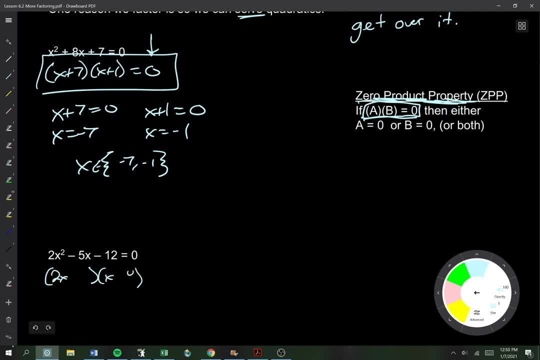 this factors. You might be somebody who likes to guess and check, where you put a 4 here and a 3 here, and a minus here and a plus here and there. that's how it factors. So if you're a guess and check guy, keep doing that. But if you're not a guess and check, 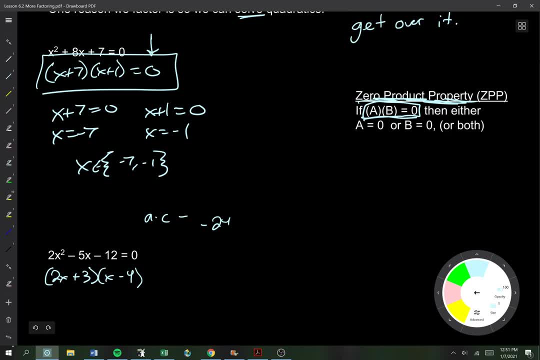 guy or gal. you can always multiply a times c. Do grouping A times c is negative 24.. So the factors of negative 24, there's a decent amount of them- are these: This pair adds to negative 5.. So I'm doing the grouping steps right now. This becomes 2x squared minus 8x.